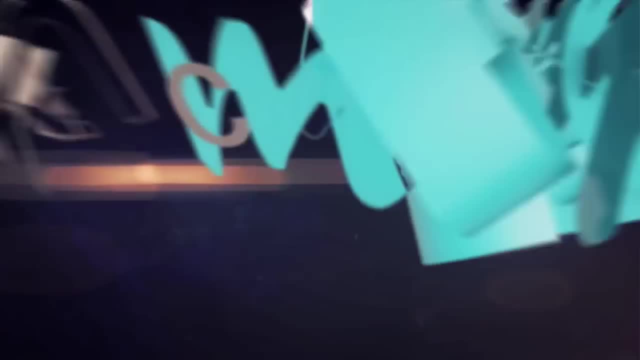 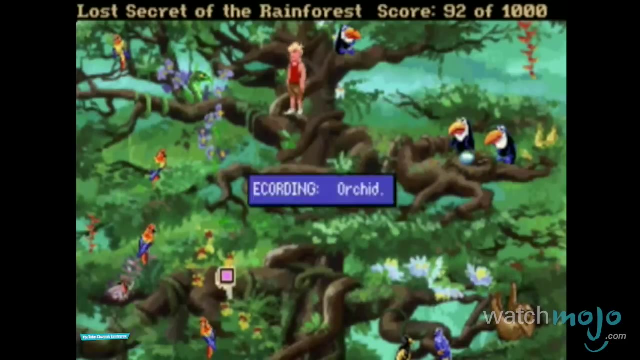 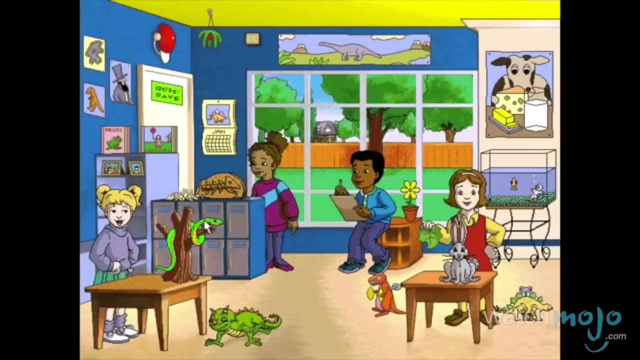 You suckers. You didn't realize that the whole time you thought you were playing a cool video game, you were actually learning: Ha, ha, ha Gosh. Dinosaurs lived for at least 165 million years. Welcome to WatchMojocom, and today we'll be counting down our picks for the Top 10 Educational Video Games. 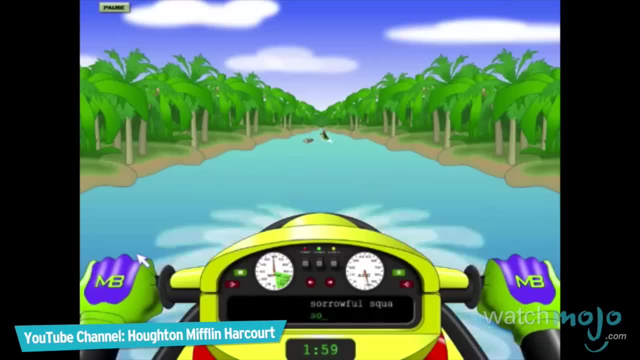 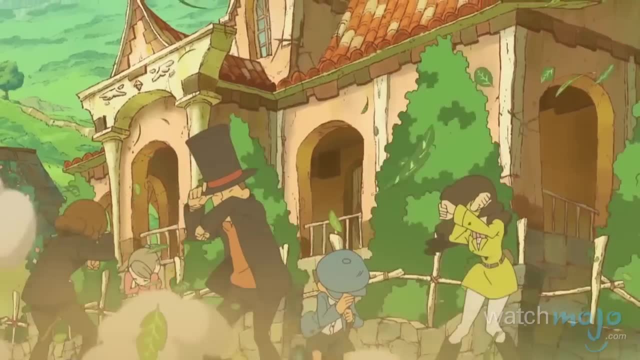 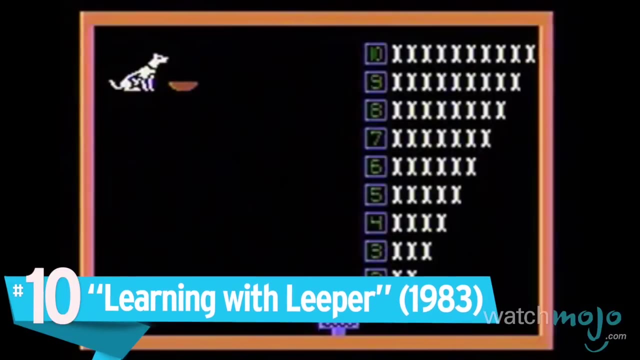 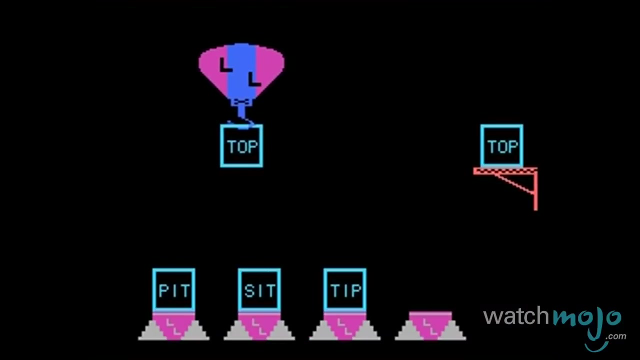 For this list, we've selected the best games that also double as educational tools. Therefore, games like Civilization and the Professor Layton series don't count, since their primary focuses aren't specifically educational. Number 10. Learning with Leaper. One of the storied PC developer Sierra's earliest titles, Learning with Leaper is a series of minigames that teaches kids basic concepts like letter and shape recognition. 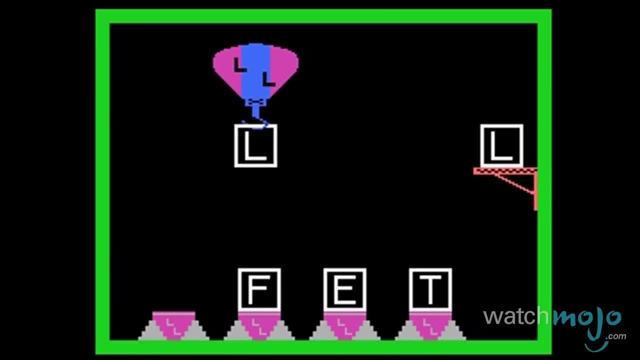 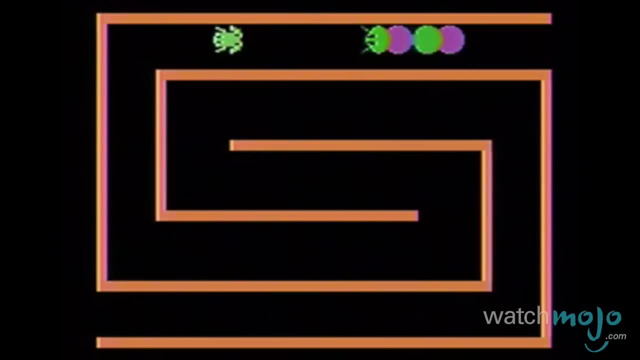 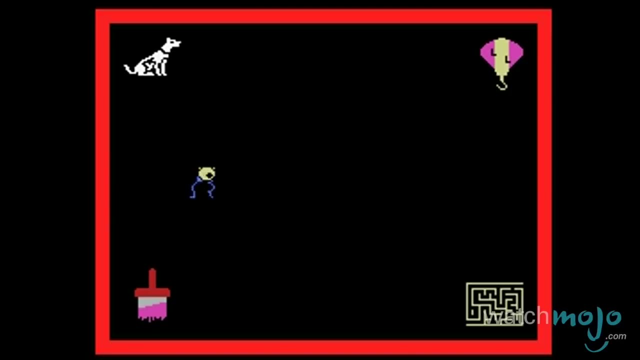 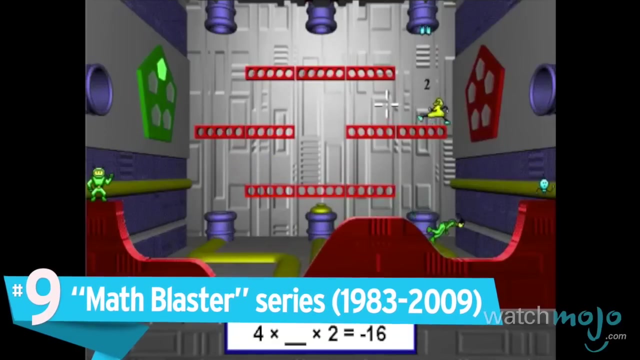 The selectable minigames show a lot of variety, from a coloring book style painting game to a randomly generated maze game, And the graphics were actually really nice and colorful for the early 80s. Number 9. Math Blaster series, Part of the broader Blaster Learning System series. 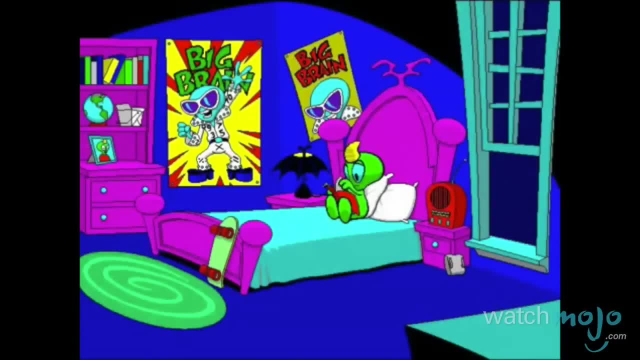 Math Blaster is an iconic part of any 80s kid's childhood. A terrible tragedy: Someone has stolen Big Brain's brain right out of his head. Combining basic arithmetic problems with fun space combat missions that take place both in the first person and in side-scrolling levels was a recipe for success. 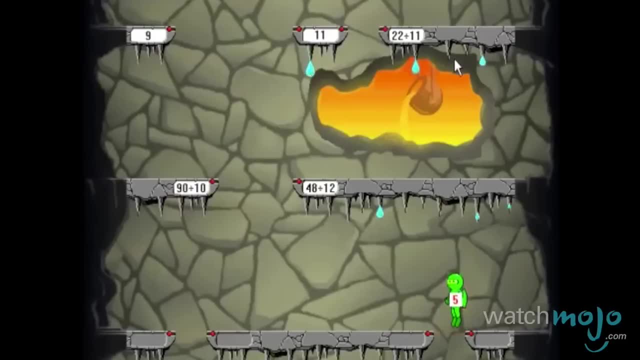 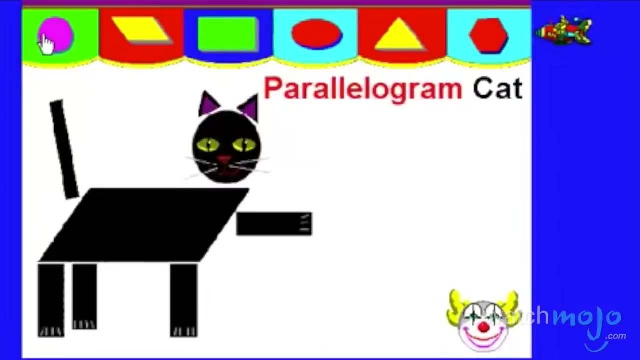 And it tricked- we mean enthralled- thousands of kids into learning their multiplication tables. Unfortunately, the quality of the later games started to go downhill as the characters and style went through transformations in an attempt to market the game to new audiences and generations. 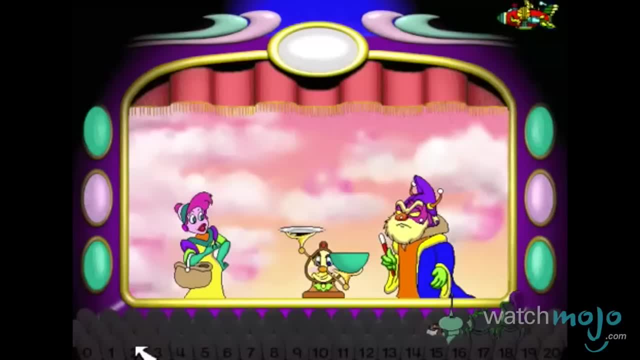 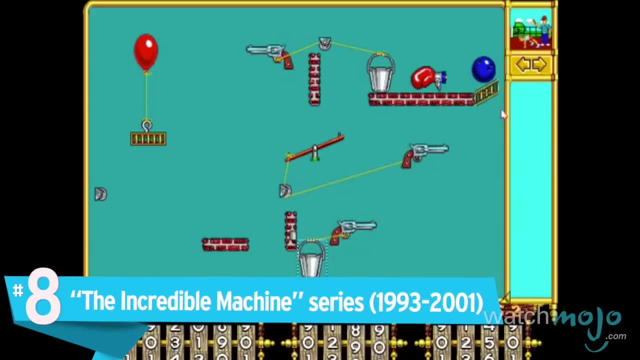 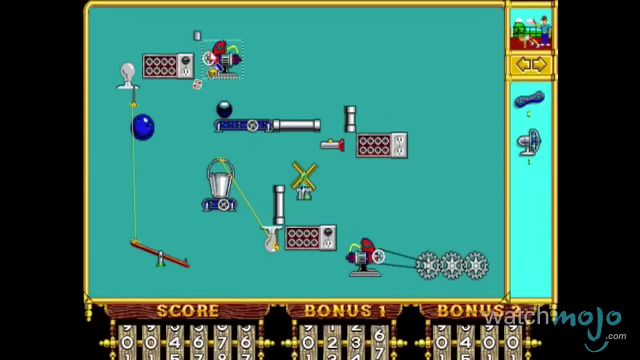 How many eggs do you think are in this bowl? Oh my, Help me guess. Two Not enough, Four, Four, Not enough. Number 8. The Incredible Machine series. Phew, Being an inventor is totally cool, especially when you're busy creating outlandish multi-faceted machines to try and solve the challenging educational puzzles in The Incredible Machine. 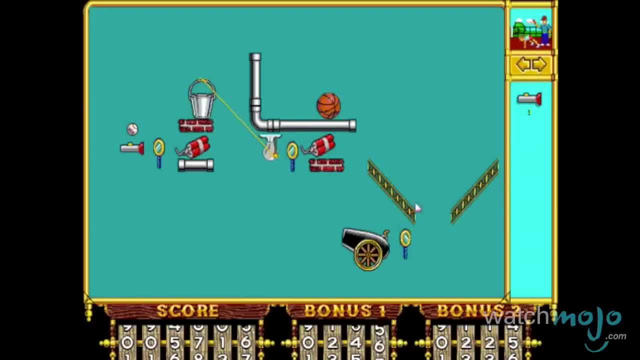 Phew, Being an inventor is totally cool, especially when you're busy creating outlandish multifaceted machines to try and solve the challenging educational puzzles in The Incredible Machine, The Incredible Machine, series U tempo, The Incredible Machine made physics and problem solving fun. 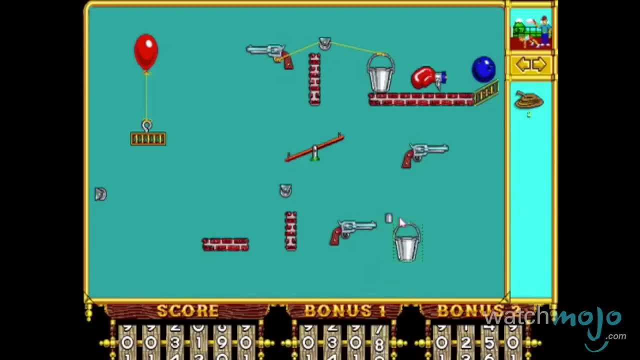 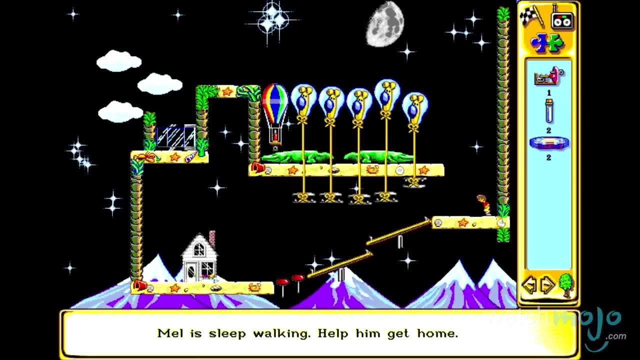 as you really had to use your brain to figure out the best way to solve the objectives in each level. The Incredible Machine series. Throughout the years, the series didn't change all that much, but that's only because the fundamental game was a perfect learning tool for players of all ages. 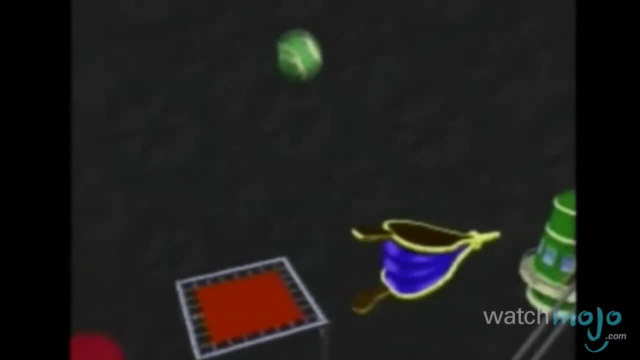 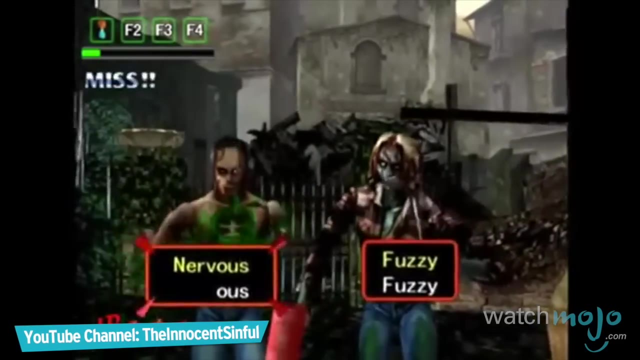 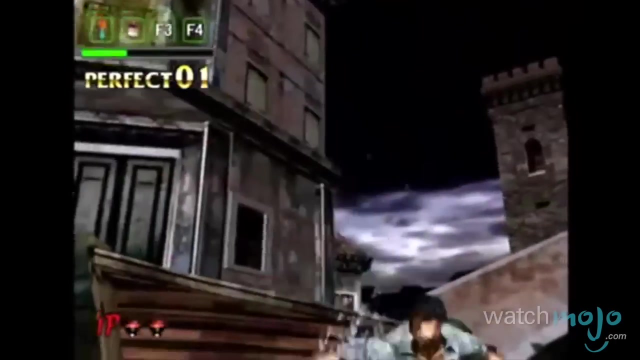 The 되яявер, The One, The Floor, Number 7. The Typing of the Dead series. Whoever thought up the concept of combining the frenzied first person light gun, zombie, blaster House of the Dead series with a typing tool is a straight up genius. 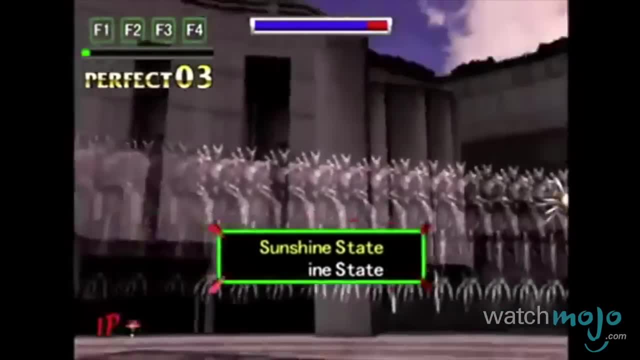 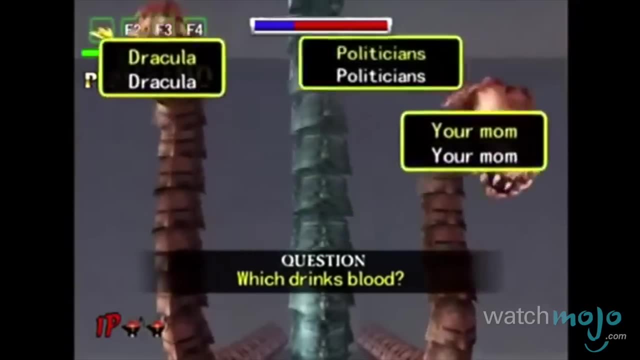 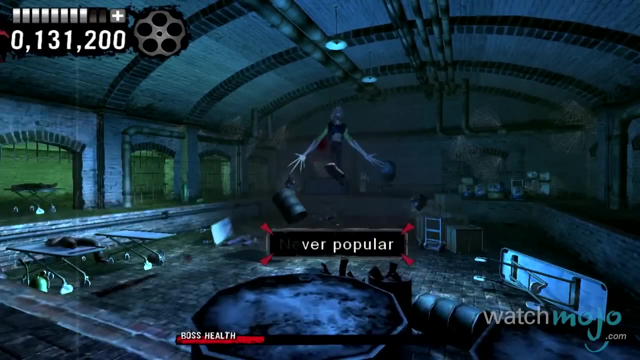 Originally bundled with the Dreamcast keyboard controller add-on, Typing of the Dead has you typing out strange sentences and zombie themed references at top speed to keep those pesky brain eaters at bay. With a subsequent re-release on Steam and new content packs coming out all the time, Typing of the Dead is still going strong as the go-to typing tutor for hardcore gamers. 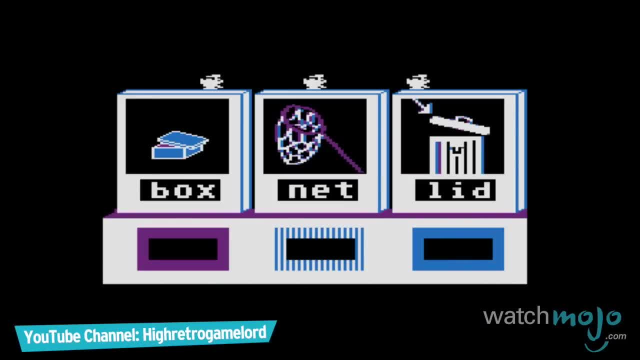 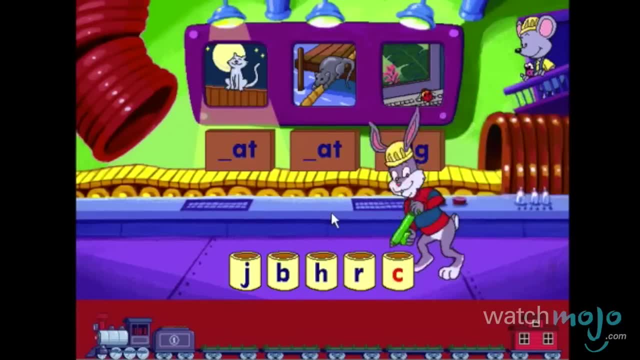 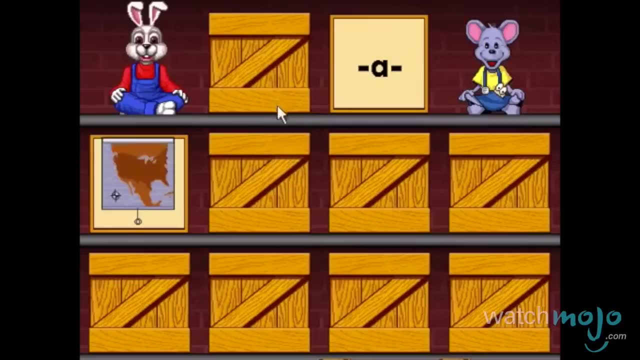 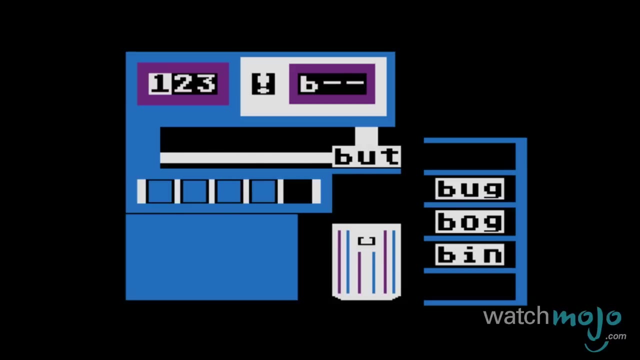 Number 6. Reader Rabbit series. Like many games on this list, Reader Rabbit is a long running series of edutainment games that has seen various transformations throughout the years. With Humble Origins as a bundle of Spelling Bee mini games for the home computer, the Reader Rabbit series has since become a giant collection of various educational games focused at different age groups, teaching basic skills in everything from math to reading. 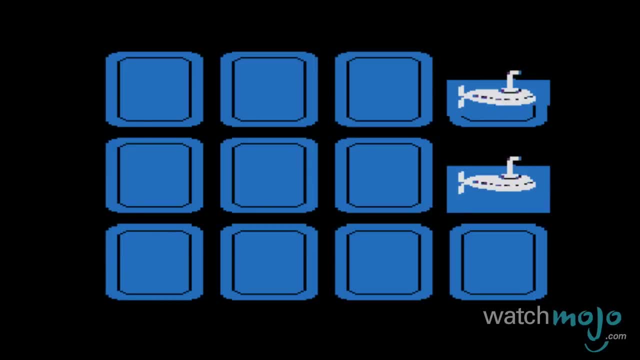 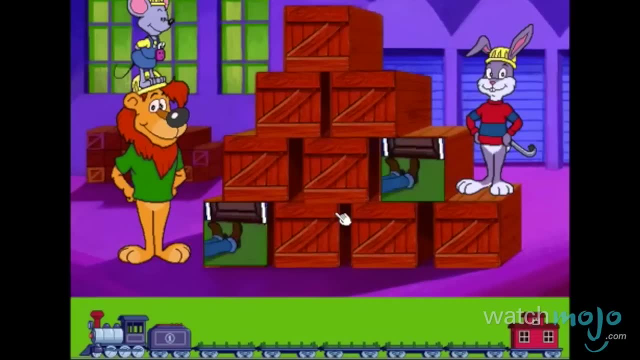 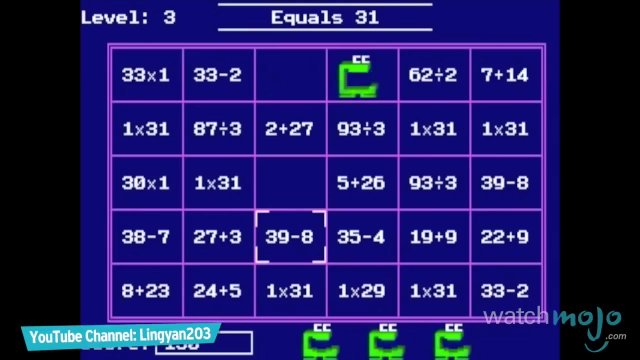 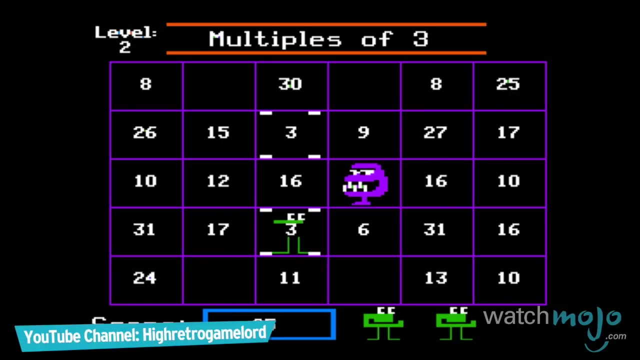 This series has won multiple awards and it helps that the characters, animation and gameplay have become more dynamic over the years. Number 5. Number Munchers: Here's a basic math equation for you. the formula for one of the most successful arcade games ever in. Pac-Man, plus a relatively basic math learning tool, equals money and a lot of smarter kids. 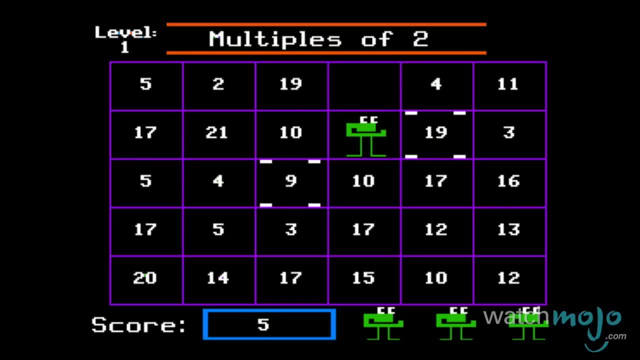 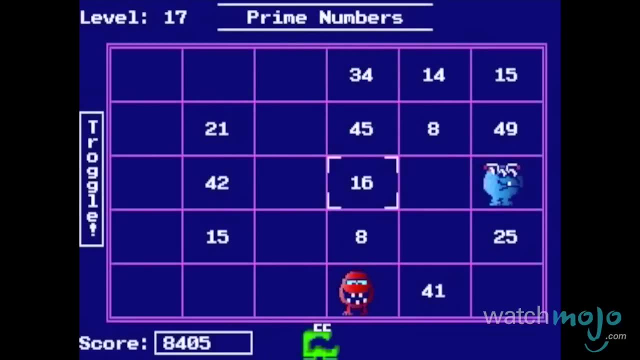 In order to move your character from one square to the next, you have to pick the square with the correct answer to the math problem at the top of the screen. all while avoiding those dastardly monsters. Plus, by incorporating a high score system, Number Munchers kept kids coming back for more. 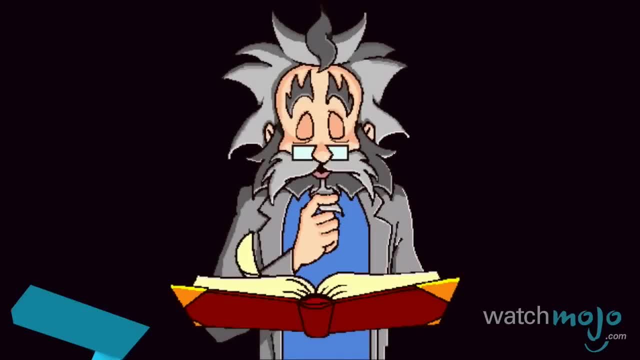 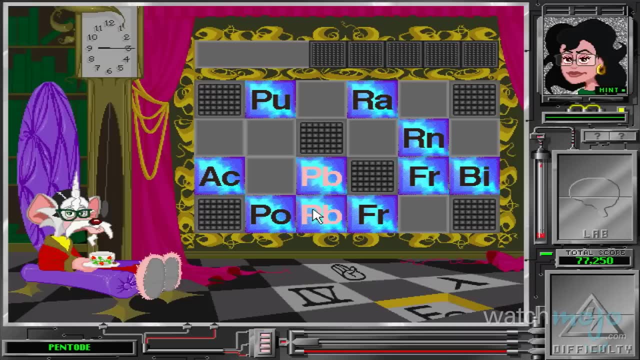 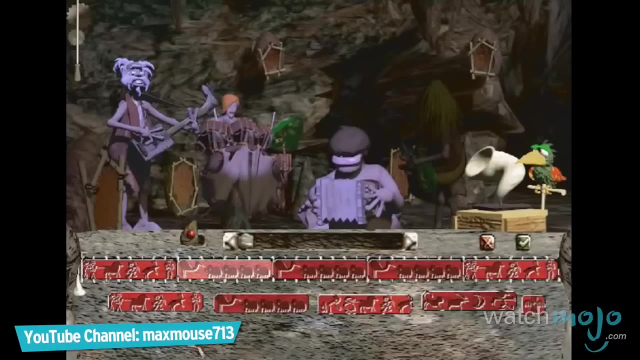 Number 4. Doctor Brain series. The long standing Doctor Brain series was one of the most successful edutainment series of the 1990s, for two main reasons. First, it broadened the scope of the subject matter in each of its entries beyond the game itself. 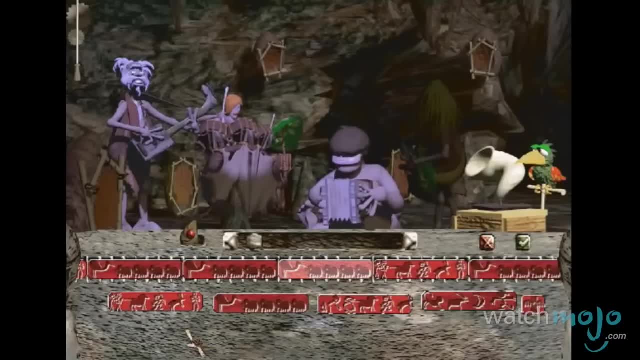 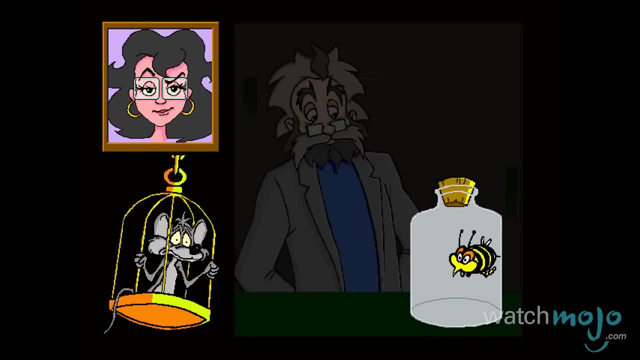 Second, it broadened the scope of the subject matter in each of its entries beyond the game itself. Instead of focusing specifically on math or spelling, Doctor Brain tried to incorporate a whole slew of different subjects through a wide variety of unique and different mini-games, from puzzles to platformers. 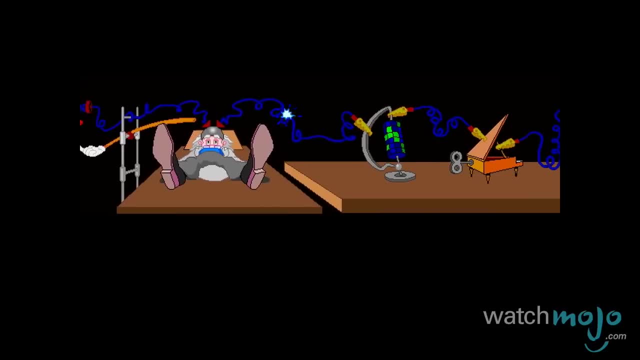 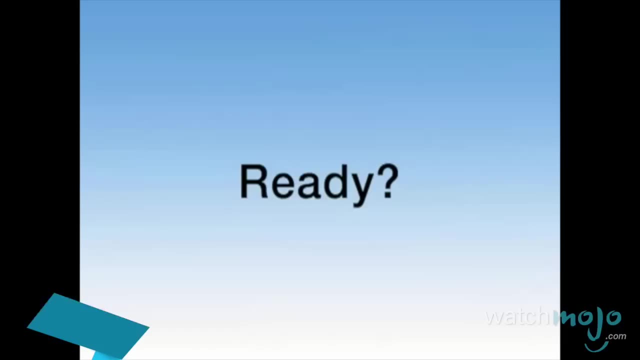 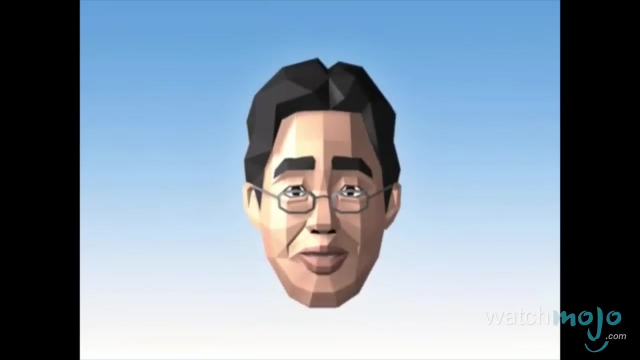 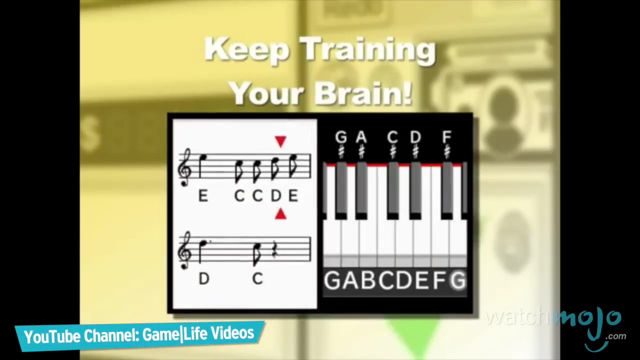 Secondly, these games were just charming as hell, filled with funny characters, lots of jokes and bright, lively graphics. Did you ever think about becoming a plumber? Number 3. Brain Age series, One of the more recent entries on this list, Brain Age was a double-edged attempt by Nintendo to both revitalize the dwindling edutainment game market and to market it more towards adults than kids. 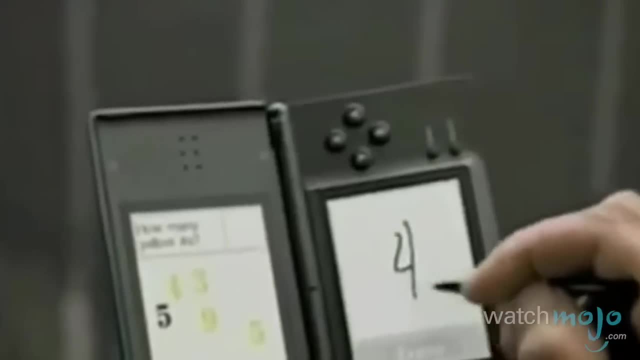 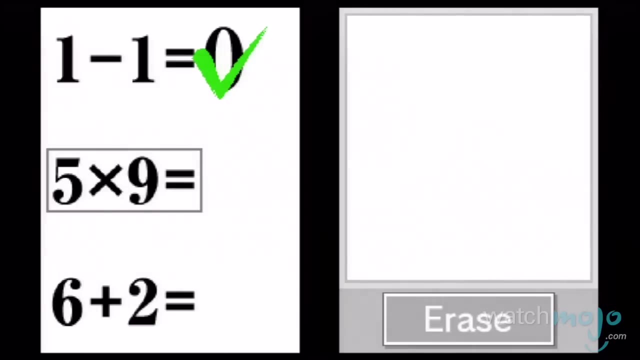 Do you need a count with your fingers? Could you stop that man? I'm trying to get some help from the flight attendant. By tracking the player's progress day-to-day as they complete the various brain teasers and mini-games, Brain Age gives players a real sense of progression as they sharpen their minds. 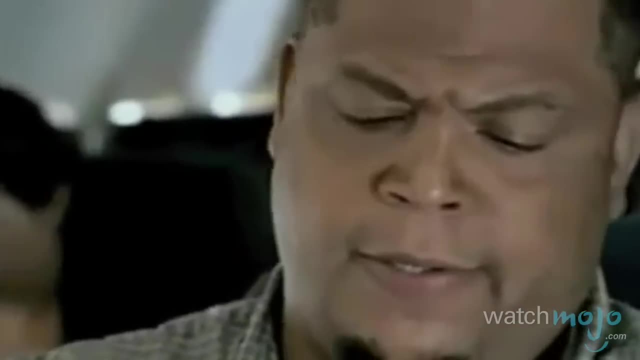 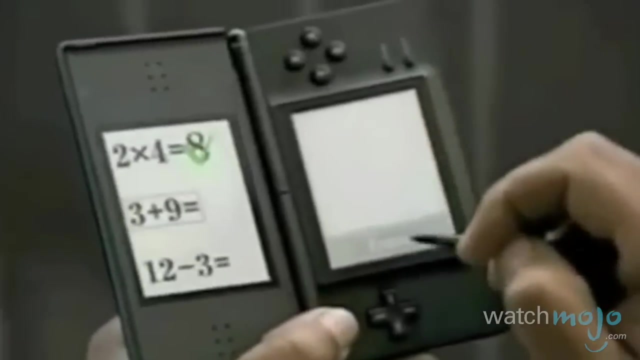 Perhaps most importantly, the Nintendo DS's stylus system was a match made in heaven for an educational tool allowing players to solve puzzles and complete mini-games quickly and efficiently. Hey, you got one. Alright, Ooh, horrible Number 2. Carmen's San Diego series. 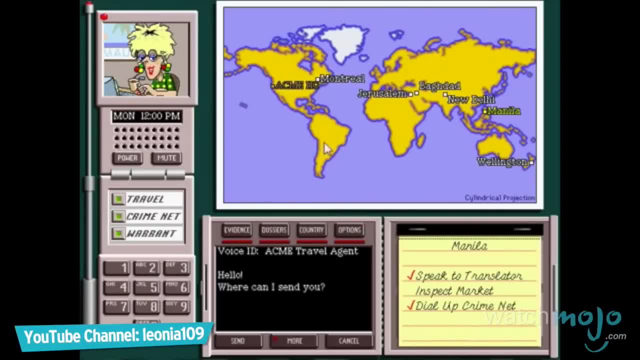 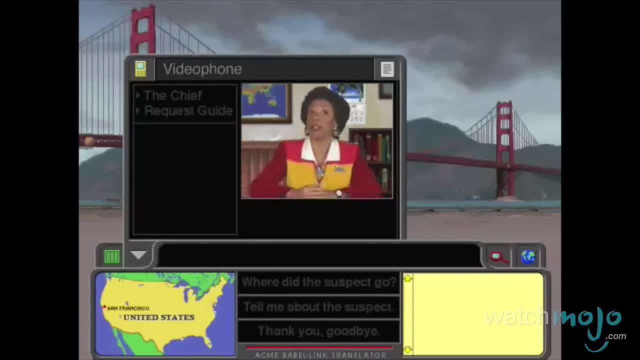 Hello, Where can I send you? Where in the world is Carmen San Diego? Well, in the late 80s and early 90s she was absolutely everywhere. I could tell you lots more, but the best way to learn a job is on the job.